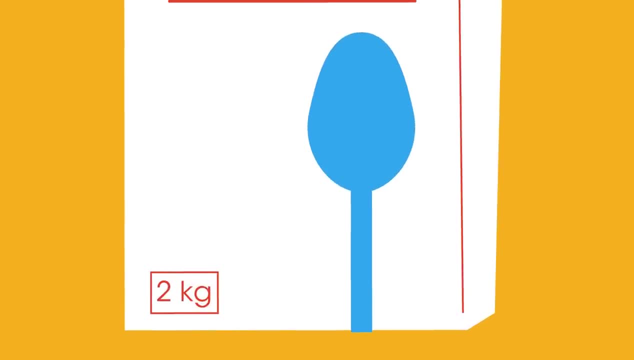 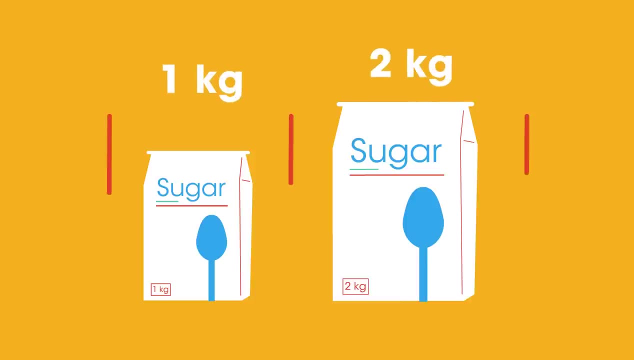 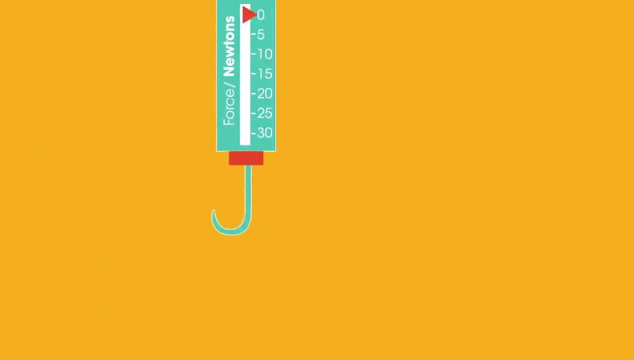 It has a mass of two kilograms. It would be wrong to say the bag weighed one kilogram or two kilograms, as weight is a force caused by gravity. To measure the weight we need a spring balance or force meter. This is a force meter or a newton. 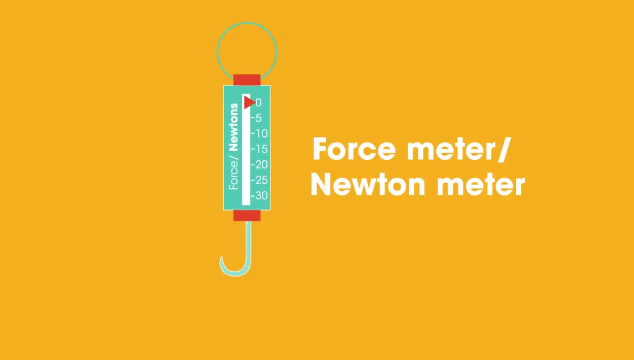 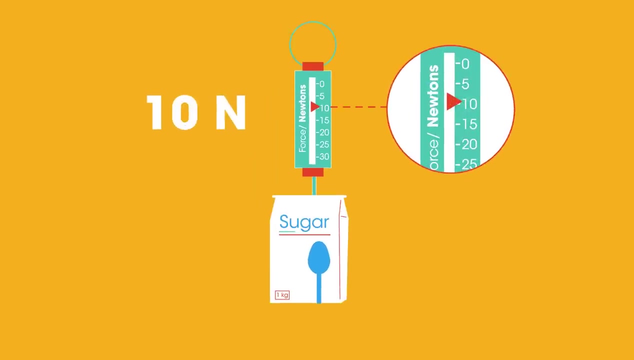 meter. It shows the weight of something hung from it. Let's add the bag of sugar: It shows the weight is almost 10 newtons. Can you remember the equation that links mass with weight? Remember: F equals MA, where F is force in newtons. 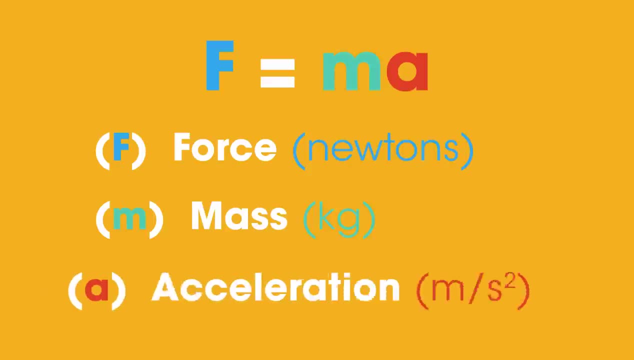 M is mass in kilograms and A is acceleration in metres per second. per second. We can rewrite this a little as: W equals MG, where W is weight in newtons and G is acceleration due to gravity On Earth. G equals 9.8 meters per second. third time: 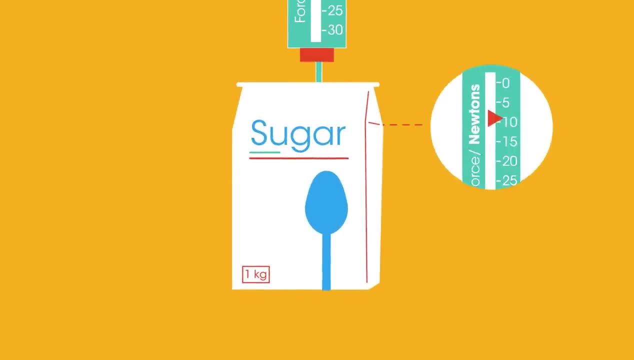 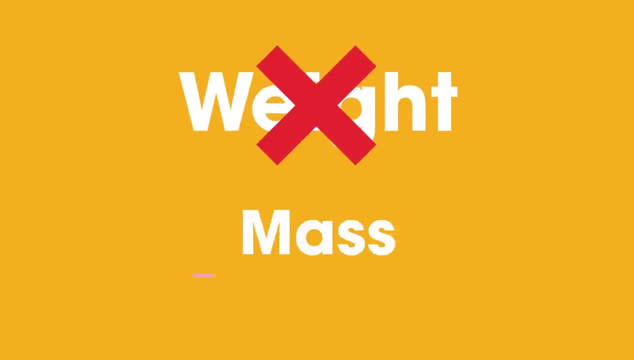 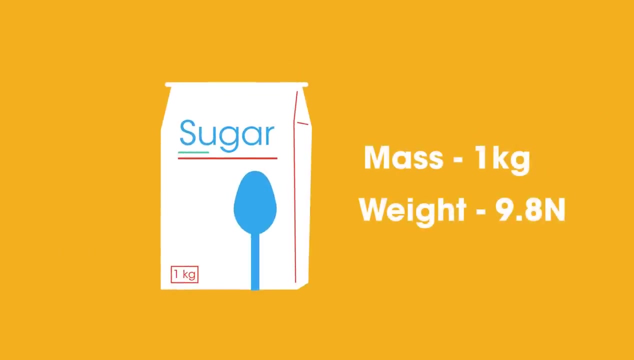 per second. so the weight of the one kilogram bag of sugar is 1 times 9.8, which equals 9.8 newtons, as the picture shows. often in everyday life we use the word weight when in fact we mean mass. the bag of sugar has a mass of one kilogram, but a weight of 9.8 newtons. 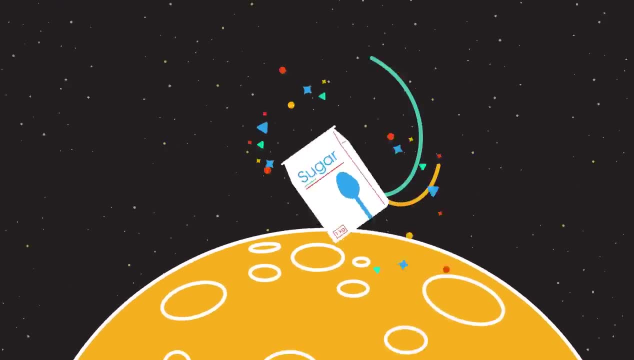 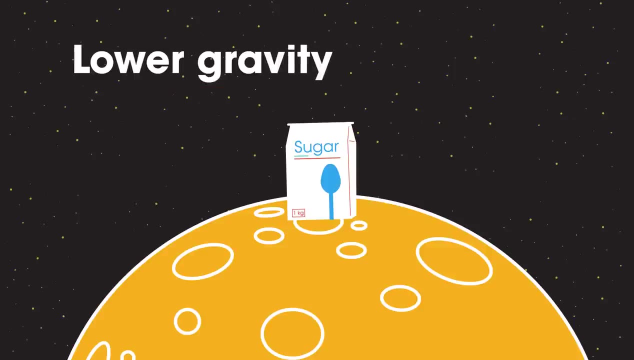 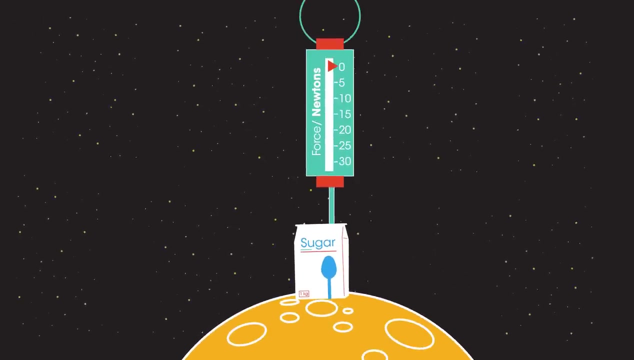 now let's take this bag of sugar to the moon. the moon is much less massive than the earth and so has a lower gravity. on the moon, g is only 1.6 meters per second. per second, see how the weight has dropped compared to when it was on earth, but notice, we still have the same. 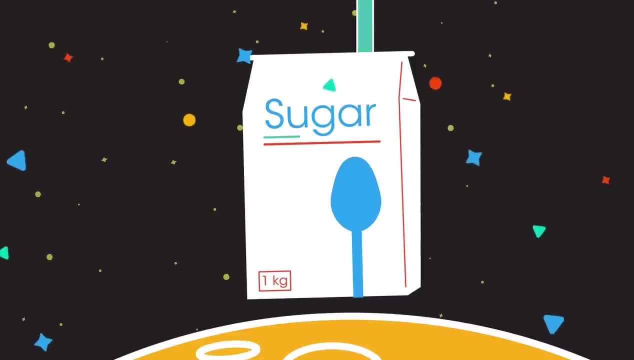 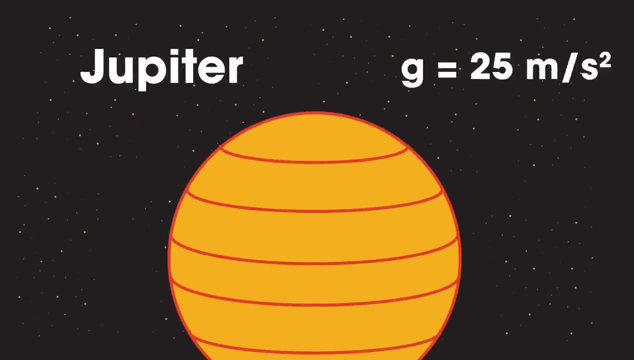 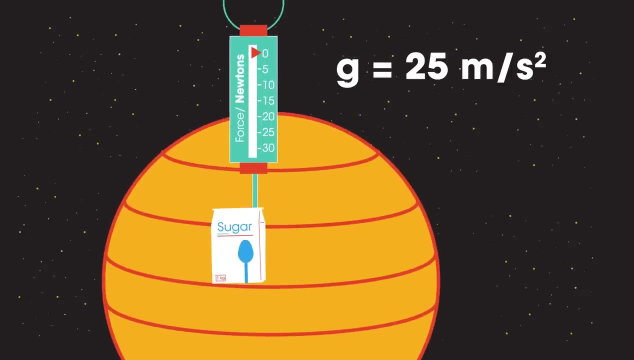 amount of sugar. there is still one kilogram of stuff. the weight has changed, but not the mass. jupiter, the gas giant, has a g value of 25 meters per second. per second, can you work out what the force meter would show for the bag of sugar here, assuming there was a? 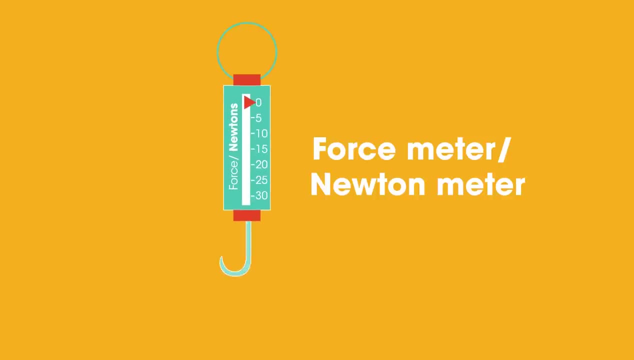 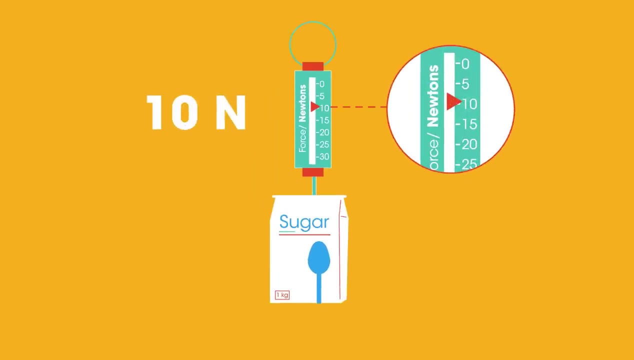 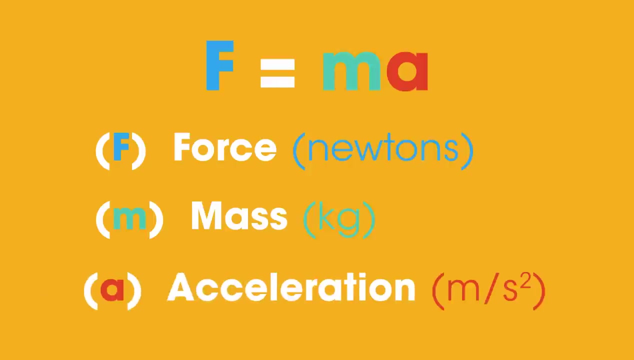 meter. It shows the weight of something hung from it. Let's add the bag of sugar: It shows the weight is almost 10 newtons. Can you remember the equation that links mass with weight? Remember: F equals MA, Where F is force in newtons, M is mass in kilograms and A is acceleration in meters per second, per second. 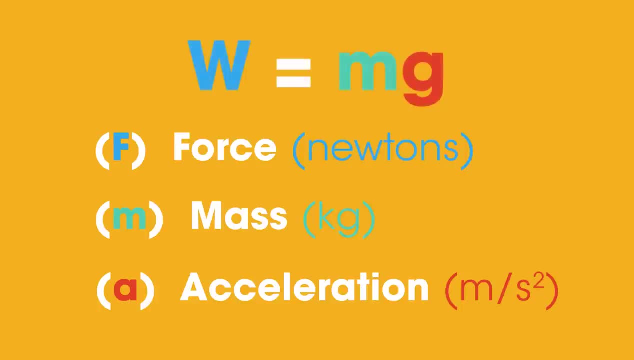 We can rewrite this a little as: W equals MG, where W is weight in newtons and G is acceleration due to gravity On Earth. G equals 9.8 meters per second On Earth. G equals 9.8 meters per second On Earth. G equals 9.8 meters per second. 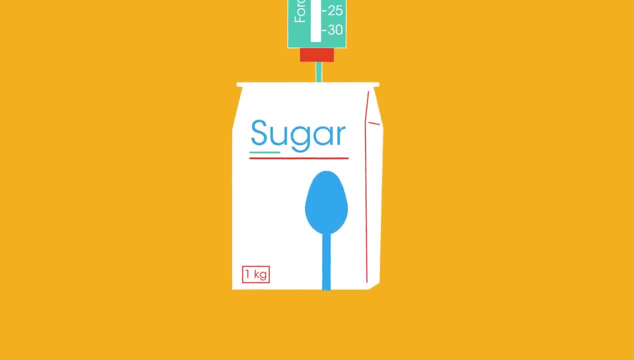 per second, per second. so the weight of the 1 kilogram bag of sugar is 1 times 9.8, which equals 9.8 Newtons, as the picture shows. often in everyday life we use the word weight when in fact we mean mass. the bag of sugar has a mass of 1. 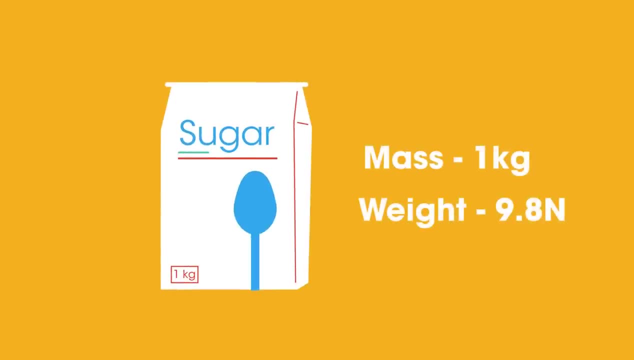 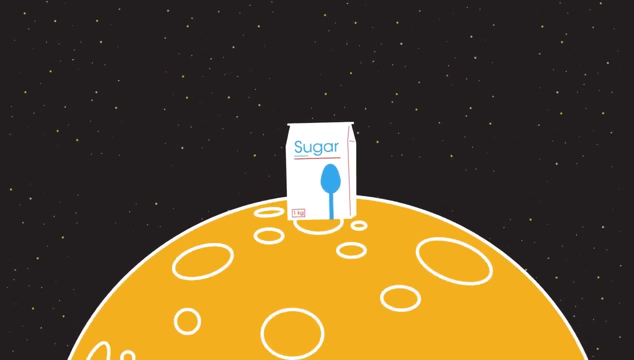 kilogram, but a weight of 9.8 Newtons. now let's take this bag of sugar to the moon. the moon is much less massive than the earth and so has a lower gravity. on the moon, G is only 1.6 meters per second. per second, see how the weight has dropped. 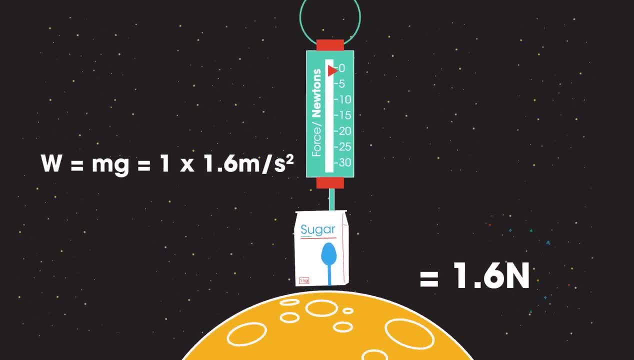 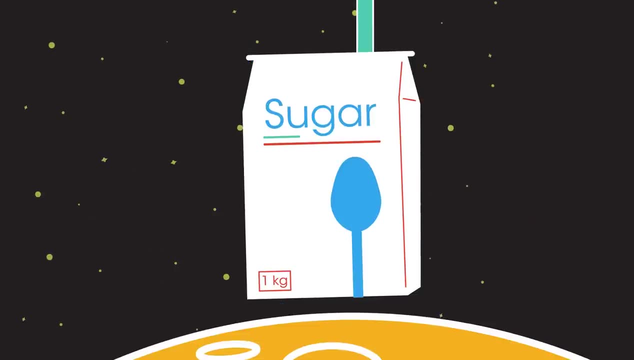 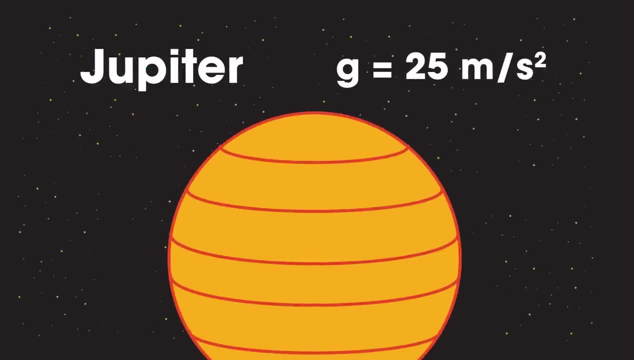 compared to when it was on earth. but notice, we still have the same amount of sugar. there is still 1 kilogram of stuff. the weight has changed, but not the mass Jupiter. again, gas giant has a G value of 25 meters per second. per second, can you work out what? 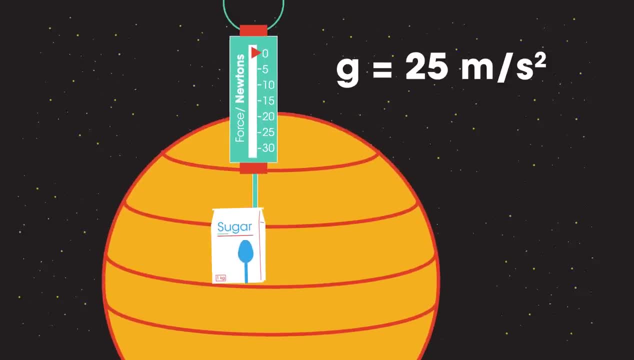 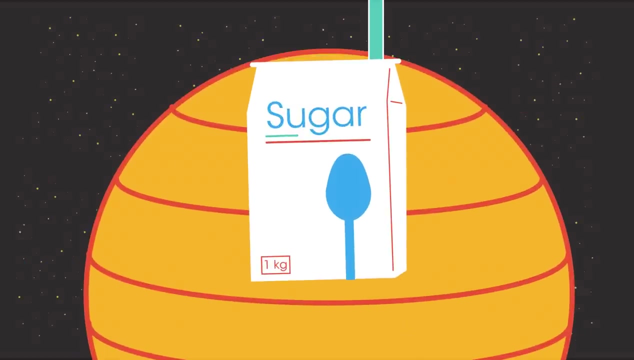 the force meter would show for the bag of sugar here, assuming there was a solid surface to stand on. the sugar now has a weight of 25 Newtons. but don't forget, we still have 1 kilogram of sugar. that hasn't changed. do you remember gravity? 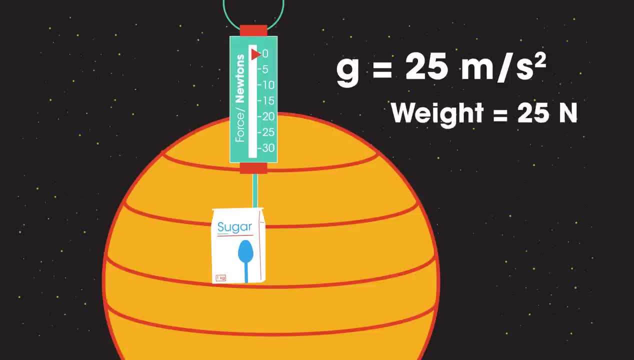 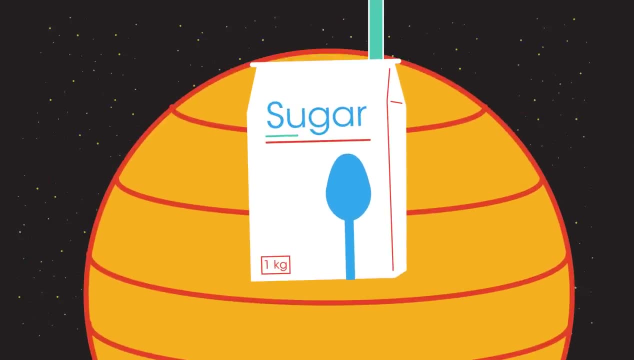 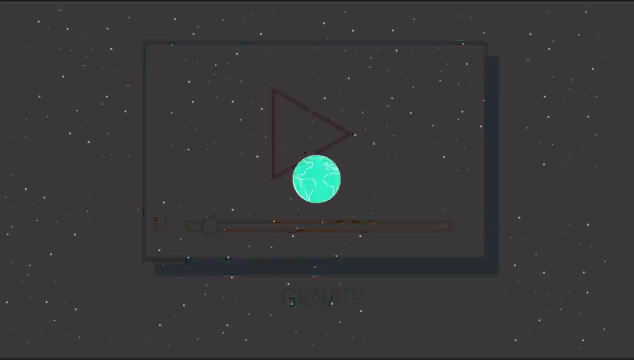 solid surface to stand on. the sugar now has a weight of 25 newtons, but don't forget, we still have one kilogram of sugar. that hasn't changed. do you remember gravity? watch this video. an object thrown away from the earth will experience a force towards the earth. 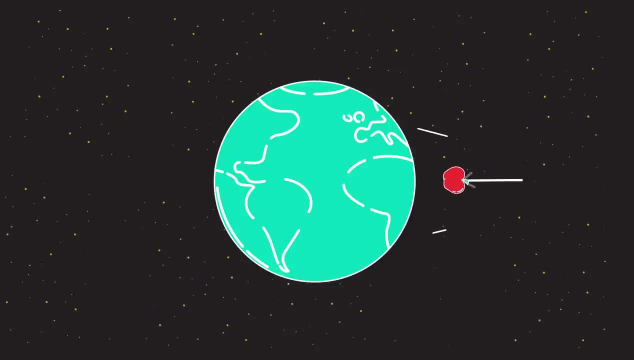 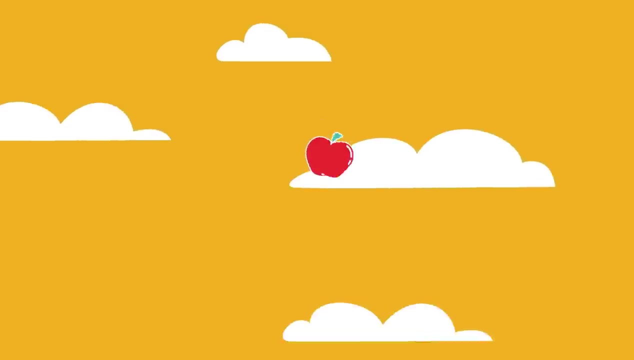 which slows it down, stops it and the object accelerates back towards the earth. this acceleration is due to the earth's gravitational force and is written as a little g. it's also known as the gravitational field strength. to stop the apple falling, so to prevent the gravitational force pulling it towards the center of the earth. 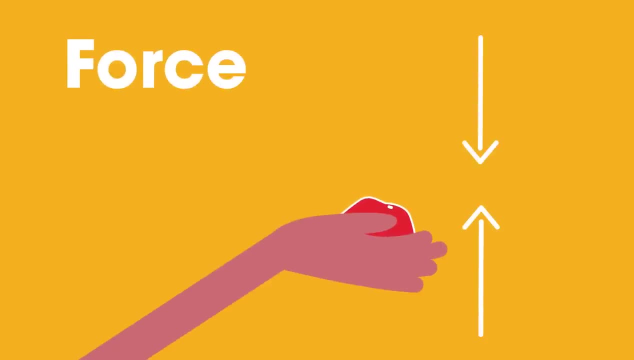 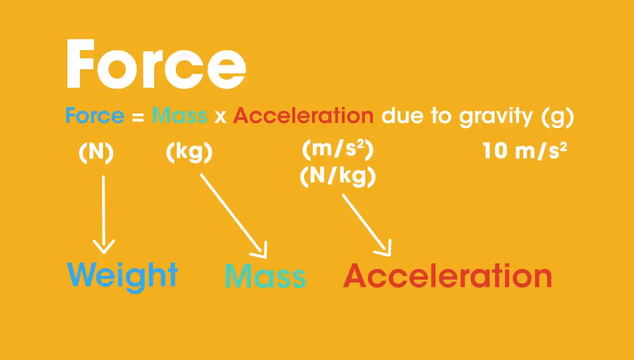 a force is needed that is equal to this gravitational pull. remember this. and on earth, g equals 9.81 meters per second per second, or approximately 10 meters per second per second. okay, back to mass and weight. remember that mass and weight are two different things. 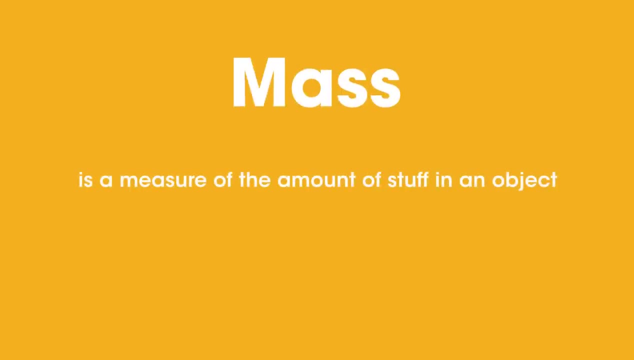 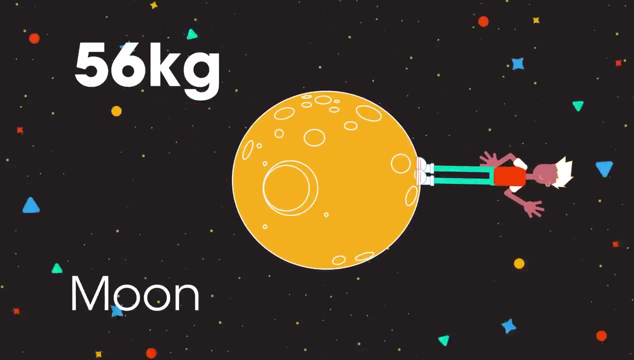 weight. mass is a measure of the amount of stuff in an object and gives a measure of how difficult it is to get moving or to stop it. it never changes. for example, my mass on earth is 56 kilograms. on the moon, i would still have a mass of 56 kilograms. 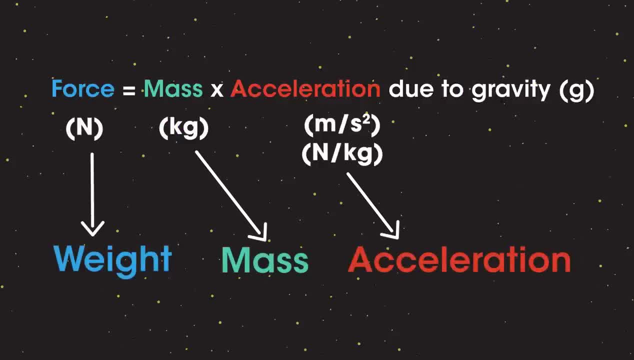 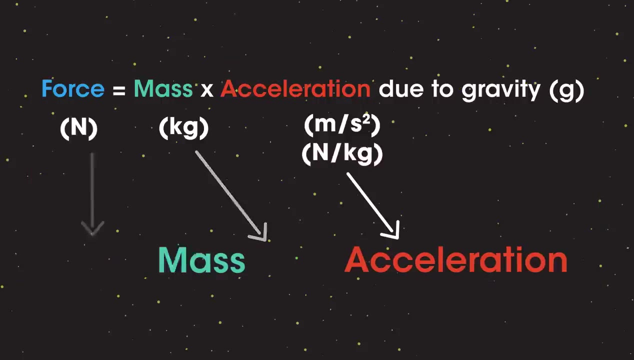 the acceleration due to the earth's gravity is measured in meters per second per second, or it can be measured in newtons per kilogram, as it's a force exerted on a unit mass. so let's now use this lovely equation to find my weight. weight is the force due to gravity, and that depends upon the masses of the two objects. 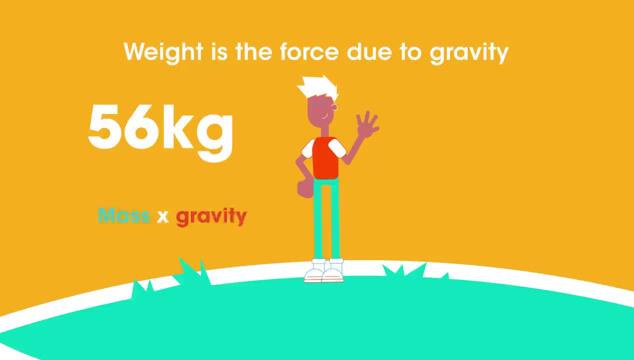 that are attracted on earth. my weight is mass times gravity, so roughly 56 kilograms times 10, which is 560 newtons. we round to 9ma mass to gravity, so roughly 56 kilograms times 10, which is 560 newtons. but what about on earth? 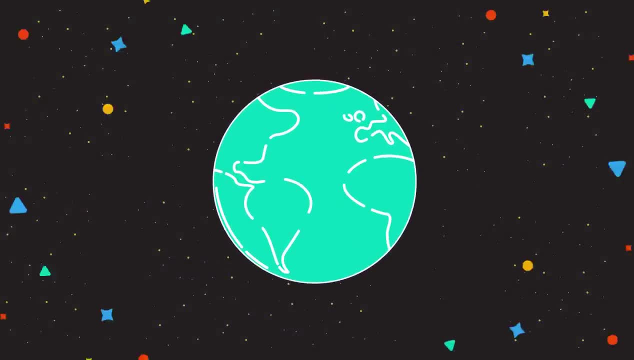 watch this video. an object thrown away from the earth will experience a force towards the earth which slows it down, stops it and the object accelerates back towards the earth. this acceleration is due to the earth's gravitational force and is written as a little G. it's also known as: 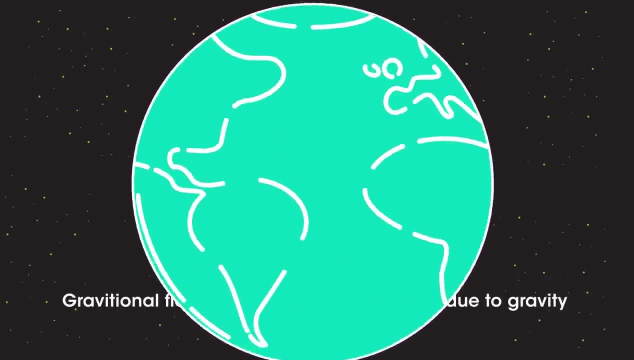 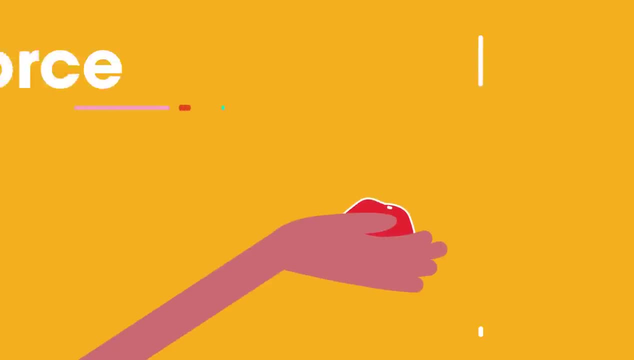 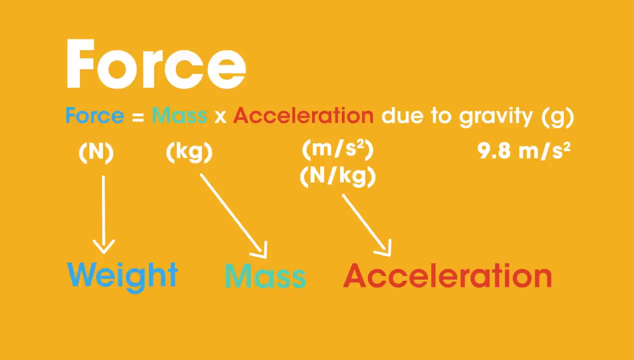 the gravitational field strength to stop the apple falling, so to prevent the gravitational force pulling it towards the center of the earth, a force is needed that is equal to this gravitational pull. remember this. and on earth, G equals nine point eight, one meters per second per second, or approximately ten meters per second per second. ok, back to mass and weight. 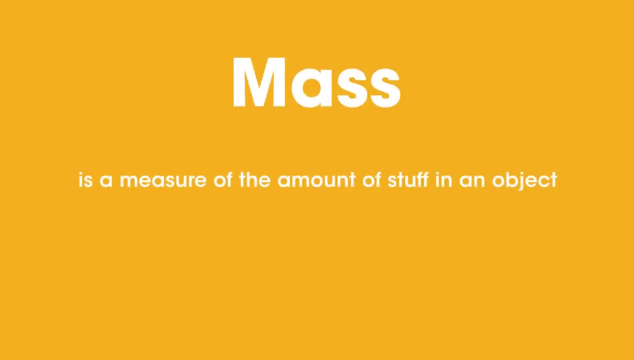 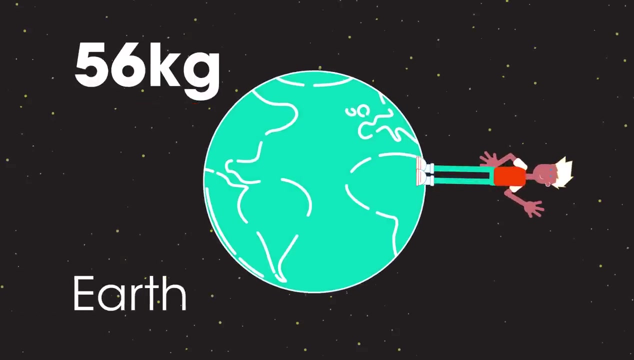 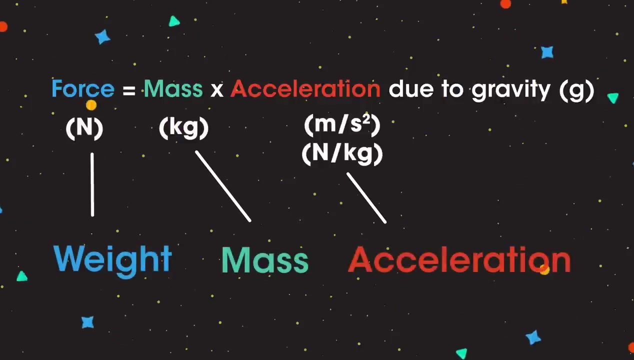 remember that mass is a measure of the amount of stuff in an object and gives a measure of how difficult it is to get moving or to stop it. it never changes. for example, my mass on earth is 56 kilograms. on the moon I would still have a mass of 56 kilograms. the acceleration due to the 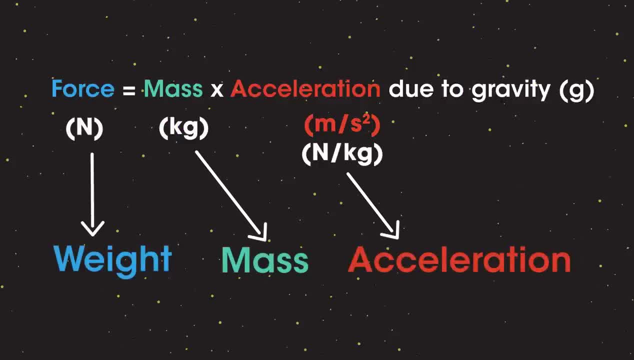 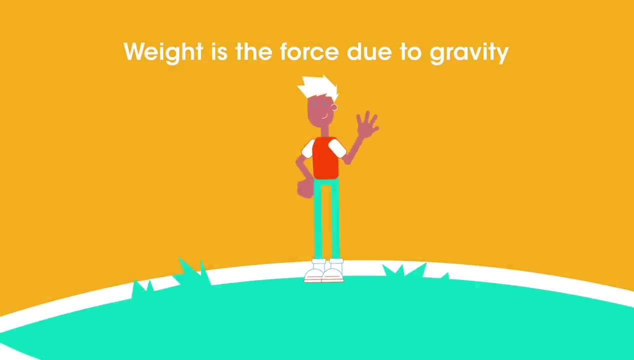 earth's gravity is measured in meters per second per second, or it can be measured in Newtons per kilogram, as it's a force exerted on a unit mass. so let's now use this lovely equation to find my weight. weight is the force due to gravity, and that depends upon the masses of the two objects that are. 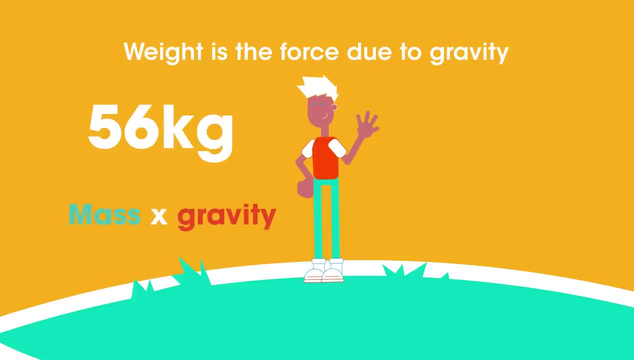 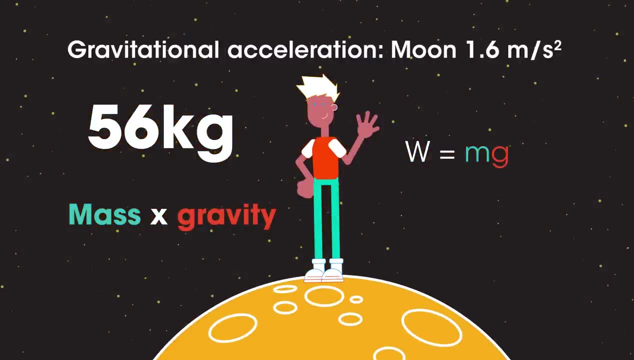 attracted on earth. my weight is mass times gravity, so roughly 56 kilograms times 10, which is 560 Newtons. but what about on the moon? the gravitational acceleration on the moon is only 1.6 meters per second, per second. I hope you got 89.6 Newtons, so you would feel very light on the moon. and if you,